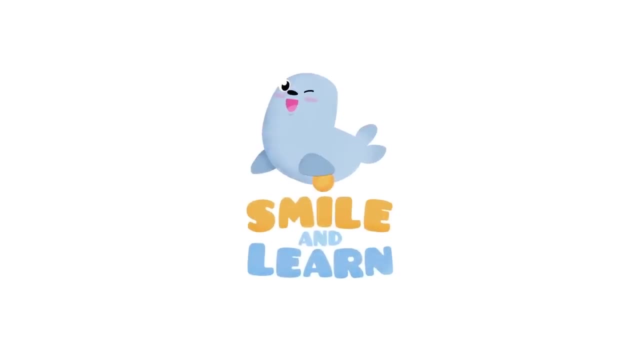 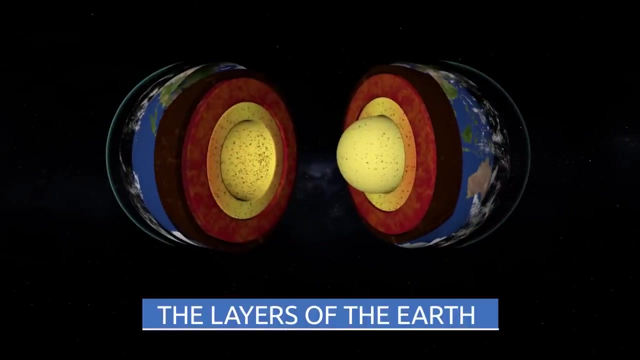 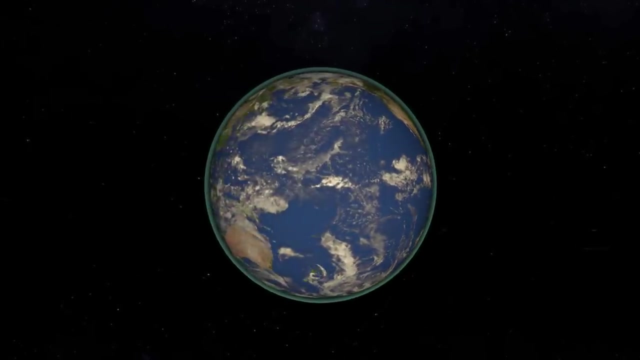 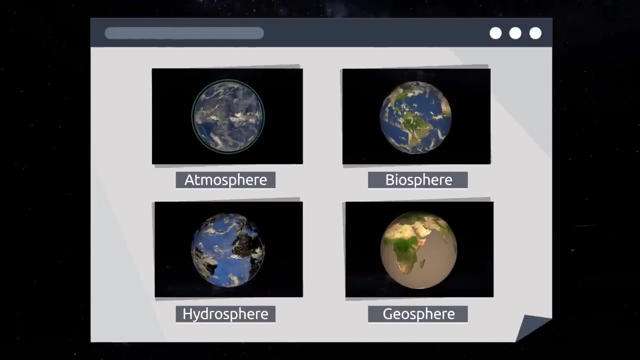 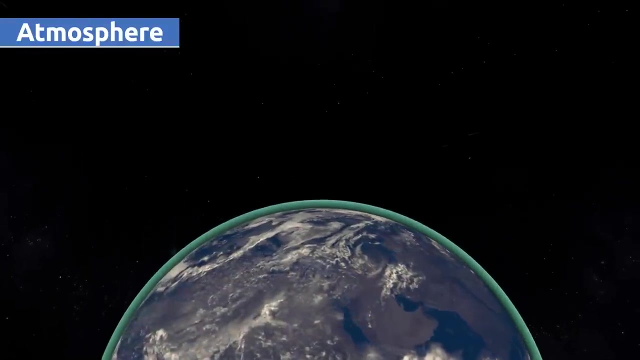 Today, we are going to learn about the layers of the Earth. The Earth is formed by four different layers. These are the atmosphere, the biosphere, the hydrosphere and the geosphere. The atmosphere is the outer layer that surrounds the Earth. It is formed by gases that protect. 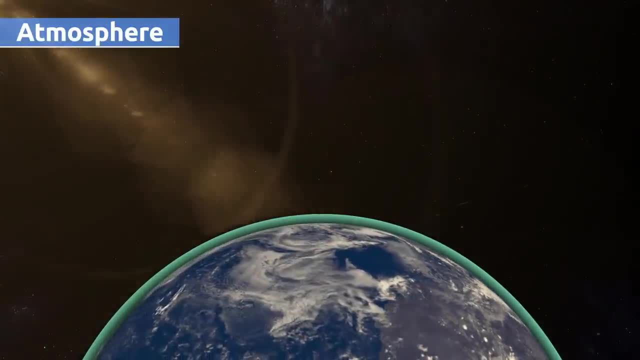 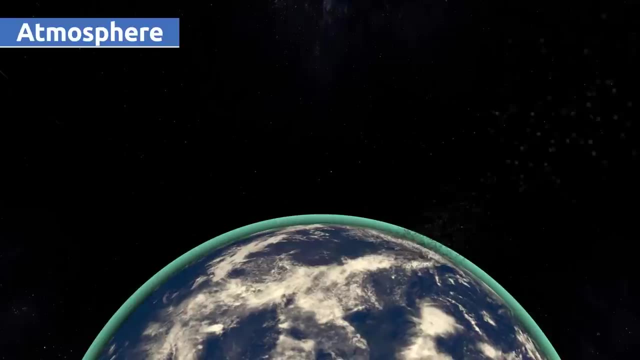 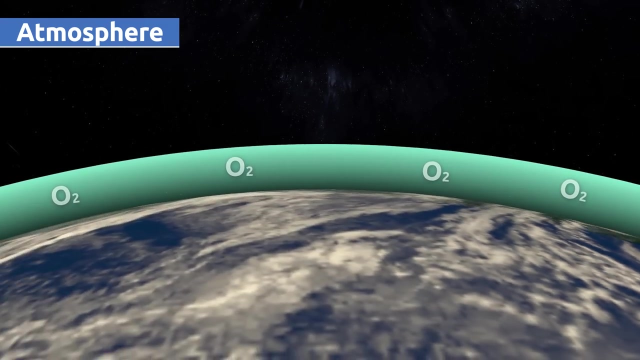 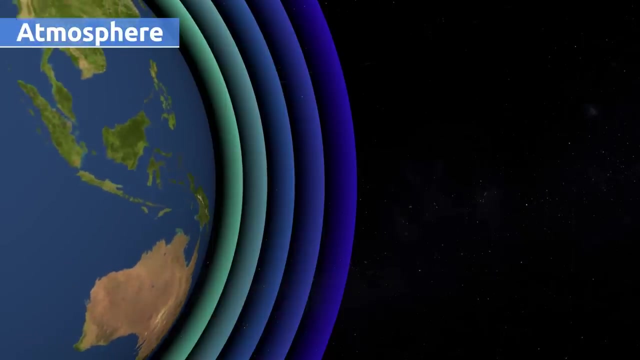 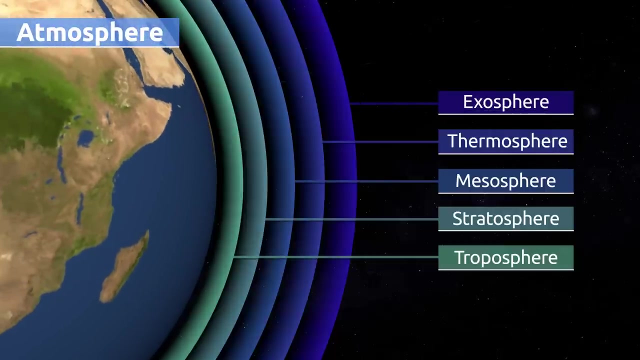 the planet from outer space, dangers like solar flares or small objects flying in space. Oxygen, that is an essential element for life, is found in this layer. The atmosphere is divided into five main layers: The troposphere, the stratosphere, the mesosphere, the thermosphere and the exosphere. 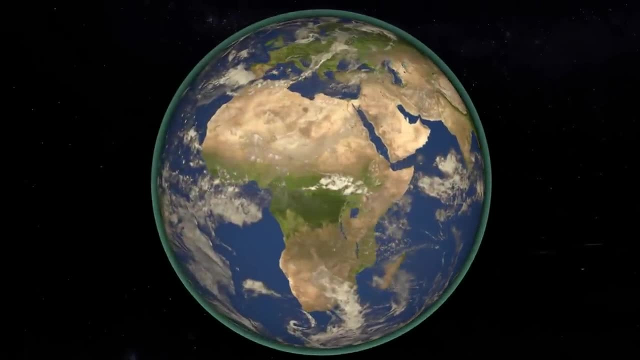 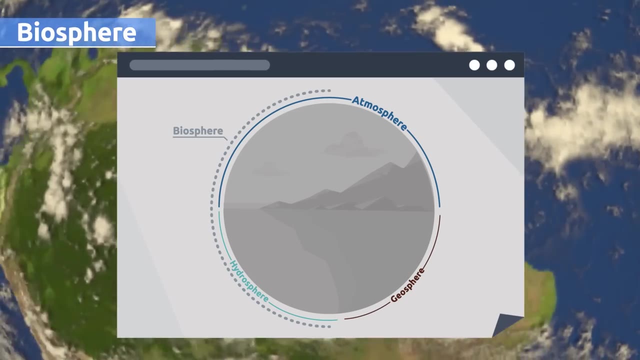 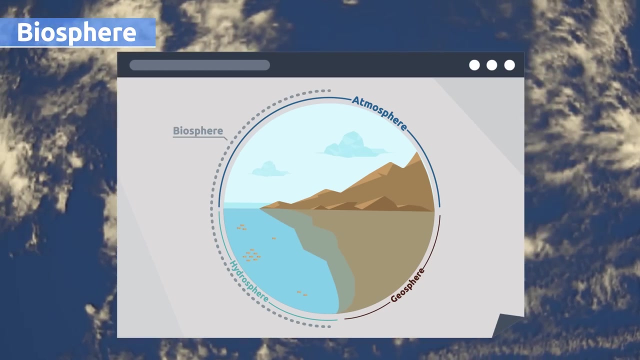 As we reach the surface of the Earth, we find two different layers: the biosphere and the hydrosphere. The biosphere is made up of all living beings. This layer extends downward to the depths of the oceans and upward to about 10 kilometers over the sea level. 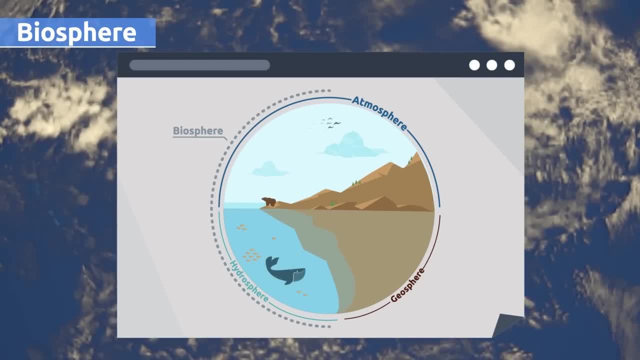 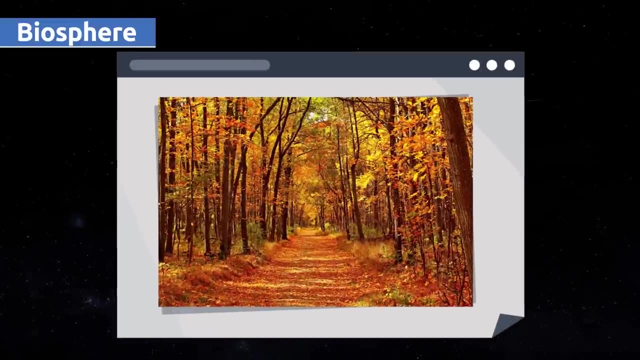 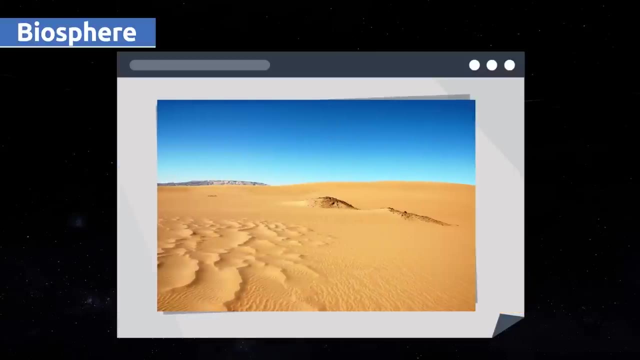 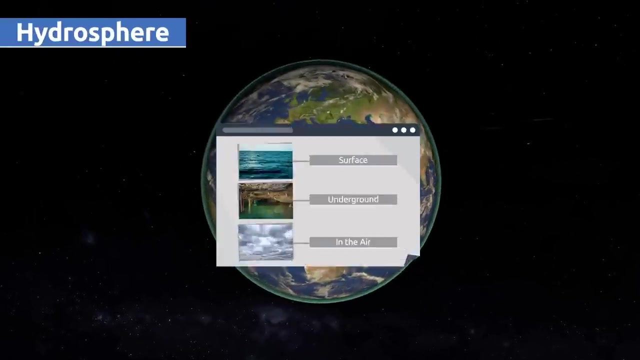 Plants, Animals, Fungi and bacteria live in this layer, together with all human beings. The biosphere is made up of several ecosystems, like the forest, the jungle, the savannah, the desert or the tundra. The hydrosphere is made up of all of the water on the Earth's surface. This layer includes 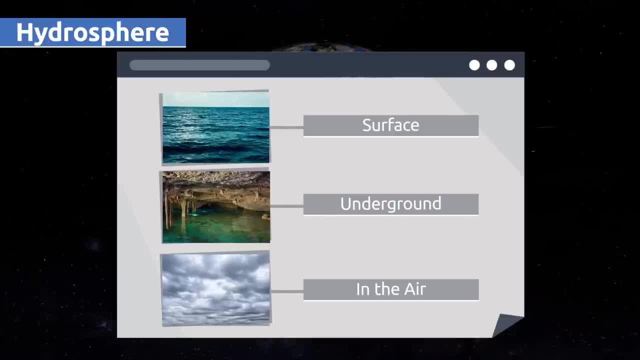 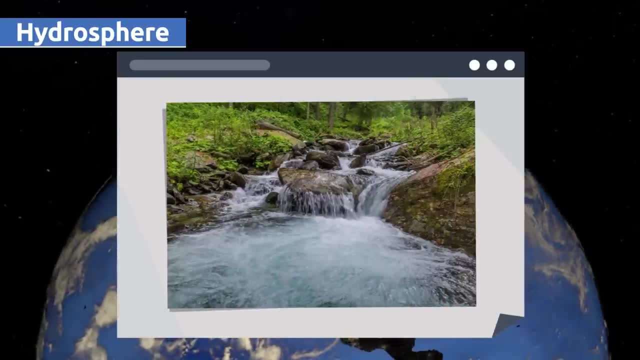 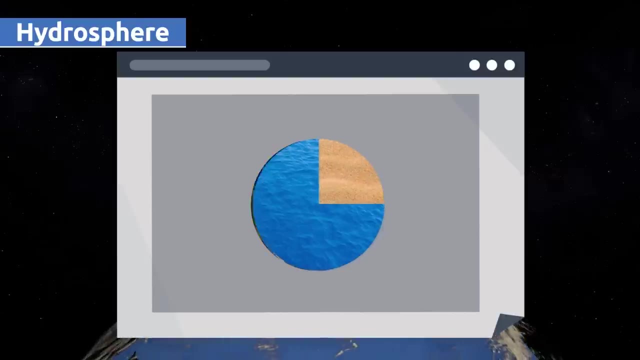 the water on the surface, underground and in the air. Water in the hydrosphere exists in three states: solid, liquid and gaseous. The hydrosphere covers three quarters of our planet. That's a huge amount of water. but 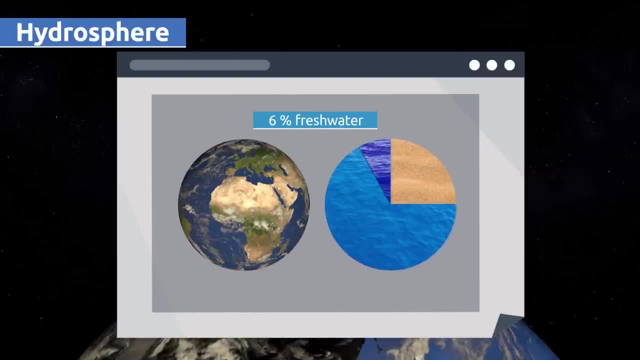 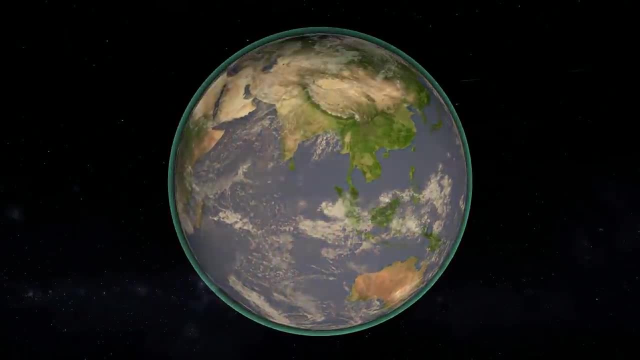 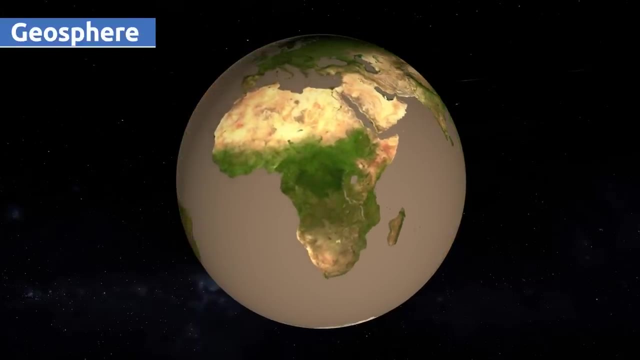 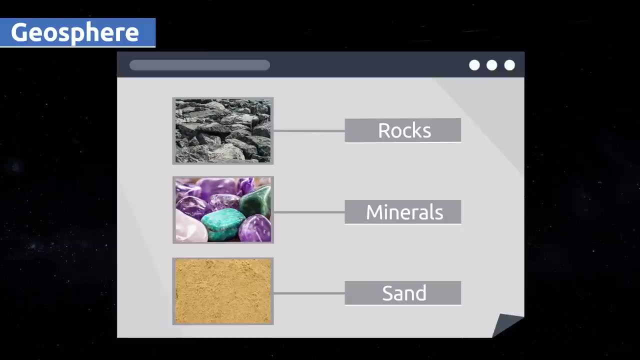 only 6% is fresh drinking water. That's why we should save as much water as we can and use it wisely. The inner layer of the Earth is the geosphere that extends from the surface to the center of the Earth. This solid ground, habitable layer is made up of rocks, minerals, sand and other materials.